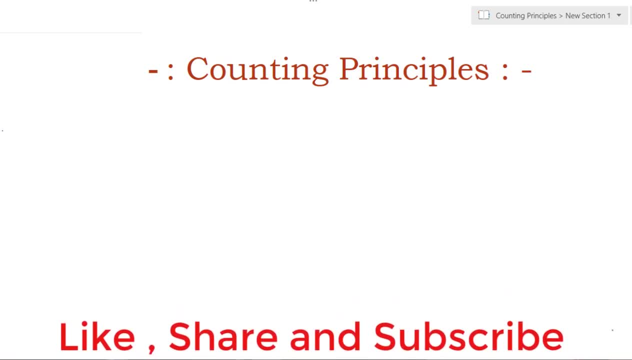 we are going to see the topic that is, a Counting Principle. Under the heading of Counting Principles we have to study various principles related with the counting. At the Counting Principles we have to see five principles of counting. Now the topic of Counting Principles. 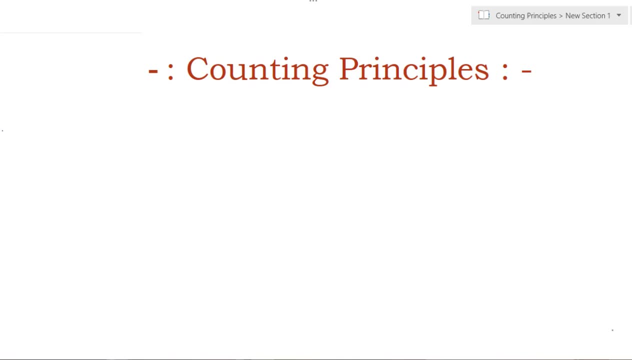 is related to Discrete Mathematics or Discrete Mathematical Structure or Discrete Structure. This point or this topic is related to many branches. Of course, it is related to BCS, BCA. In addition, MCA also has Counting Principles. This topic is included in the syllabus of the 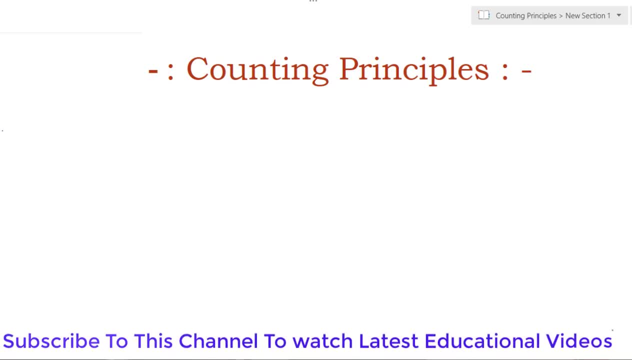 same university When we give various aptitude exams, that is of course the aptitude exam related to the software company or the MPSC, UPSC regarding or competitive examination. there too, the counting principles are also included in the counting principles. 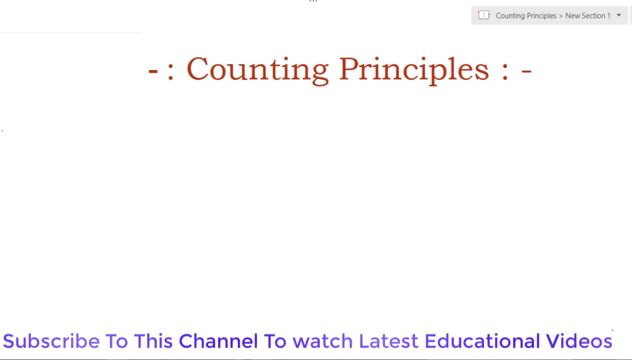 So the counting principles are also included in the counting principles. In the same way, we can use these counting principles to write some small examples within the given time limit or time bound. In short, the importance of this topic is in various fields. 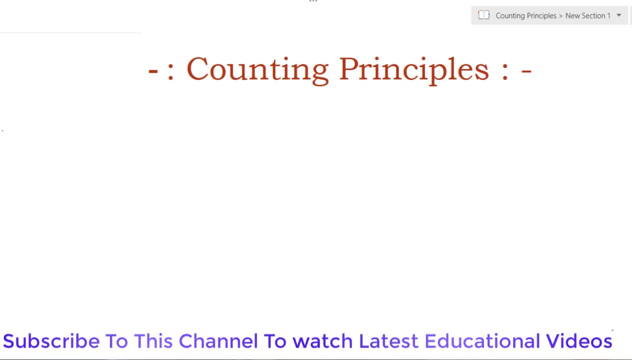 This topic have a lot of importance among the fields. So let us see Counting Principles First of all. in the Counting Principles, we have to see what is the definition of Cardinality of a Set. First we have to see what is the definition of Cardinality of a Set First we have to 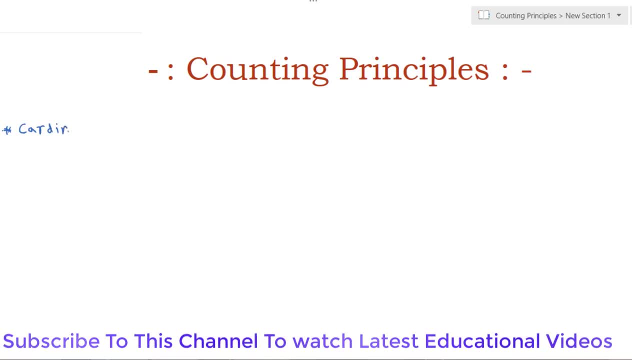 say cardinality of a set. Okay, That you know very well. These are the basic points. Now we have to see what is definition of cardinality of a set. We have a simple definition: Let capital A be a set. Then the number of elements: very simple concept: The number of elements. 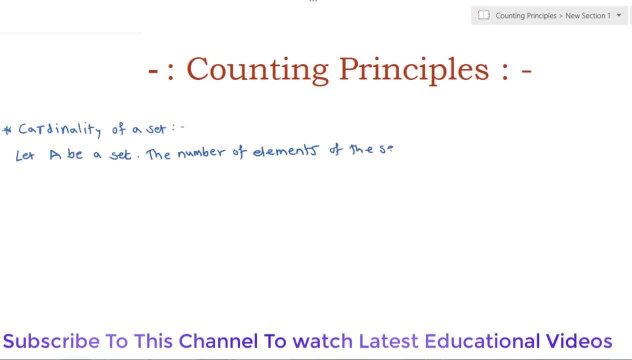 of the set capital A, of the set capital A is called as cardinality. It is called as a cardinality, is called as a cardinality of a set capital A, Of a set capital A. Very simple definition: Let capital A be a set Capital. A is one thing. Then the 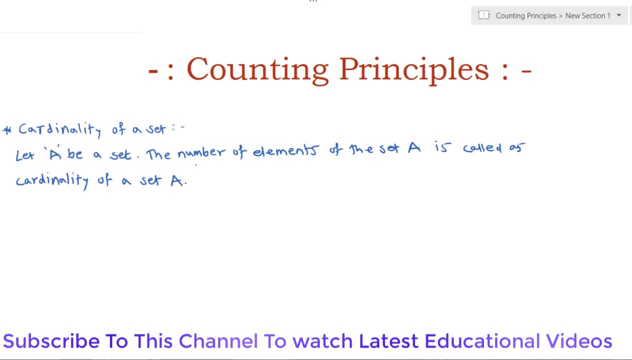 cardinality of set A means what is Number of elements? Okay, Very simple concept. the number of elements of the set in the set capital A is called as a cardinality of the set capital. A. Manje the set A madhe kiti number of elements. aayet tachi sankhya manje sthya setchi. 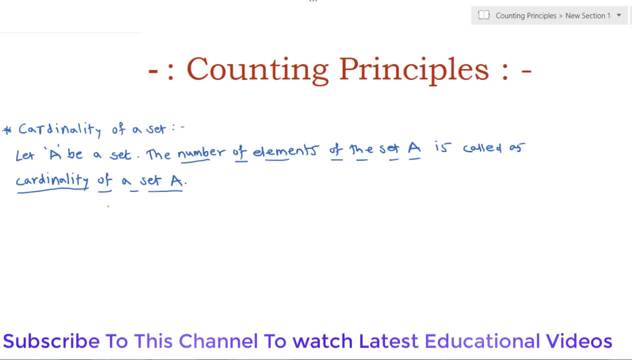 cardinality aayet. Okay, Now, symbol kaibu gaya. it is denoted by very simple concept. it is denoted by the symbol, this one, the vertical line ani madhe capital ASL. Okay, This is denoted by the symbol, the vertical line ani madhe A, and we read this as te: 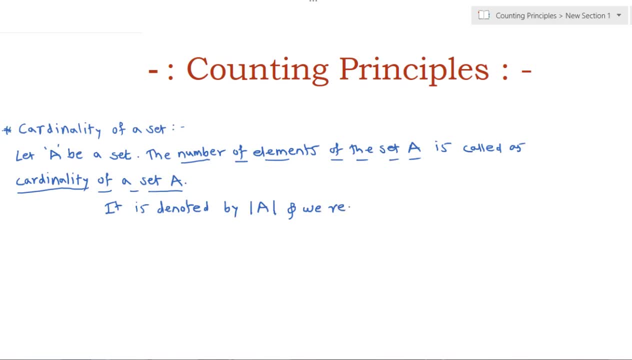 vaksa is kasa and we read this as cardinality. cardinality of set capital, A Okay, Manje, mantan hapan. cardinality of a set capital A asa mannar litana fakta hapan kailinar. 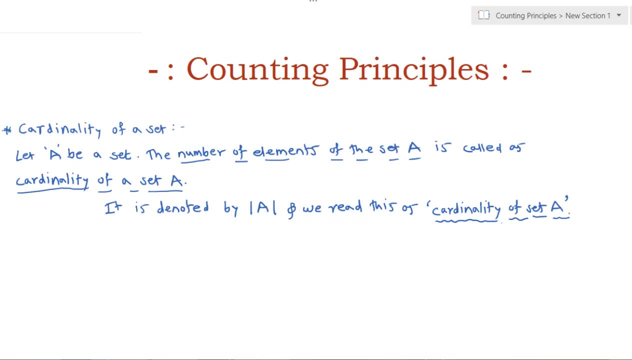 don vertical line anhi madhe A. Okay, That is denoted by the symbol don vertical line anhi madhe A, and we read this as a cardinality of the set capital A. Okay, Very simple thing. Similarly, in other books it is also denoted by: or this is ahead, symbol aayet, or it. 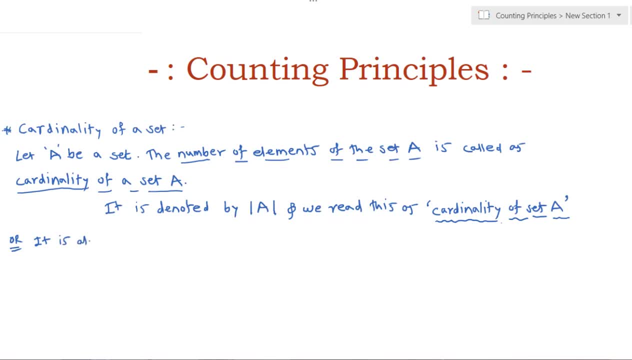 is also denoted by: or. it is also denoted by: Okay, Alright, Okay, Thank you, Thank you, Thank you. this symbol, small n, bracket, capital e, and we read this as: and we read this as: number of elements definition. 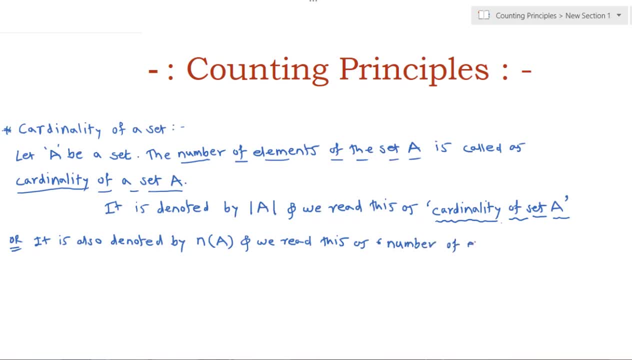 number of elements in the set in the set capital a. okay meaning, if this is written as n of a, then when we read n of a, then when we read number of elements in the set capital e, that is, number of elements of the set capital a, we will read like this: 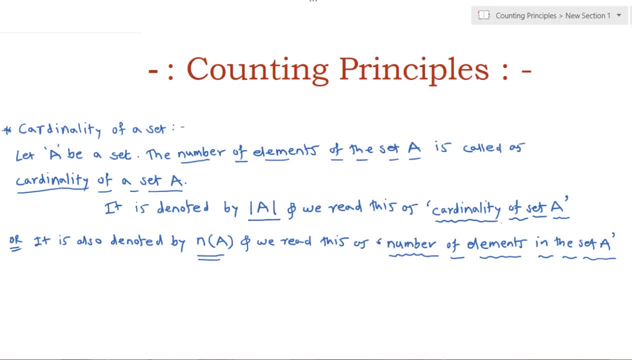 we will read like this: cardinality of this set a, and and and and n of A. we will find the number of elements of the set capital A for number of elements in the set capital A. Now, cardinality is an important concept because we have to look. 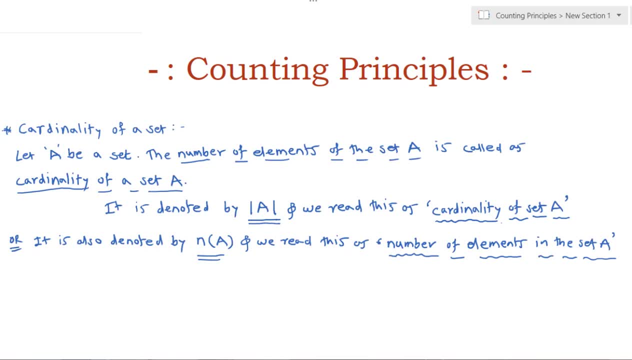 at the counting principle. Counting means: wherever there is a count, wherever there is a measurement there, we can definitely use the counting principle For that. counting means number of numbers. number of numbers means cardinality. Therefore, the first definition of this topic is the cardinality of a set A. What is the simple definition? The number. 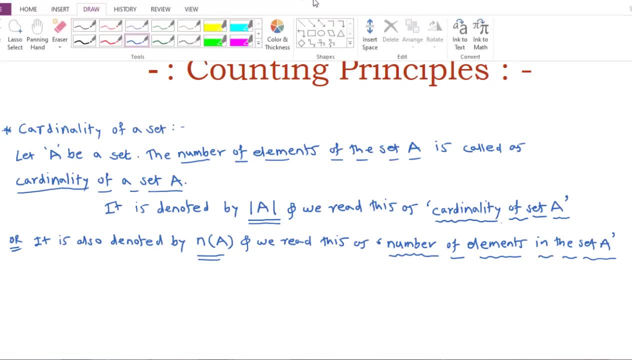 of elements in the set capital A is called as a cardinality of the set capital A, and it is rooted by the symbol this one, and we read this as a cardinality of the set A. Similarly, it is also rooted by the symbol N of A, and we read this as a number of elements in the 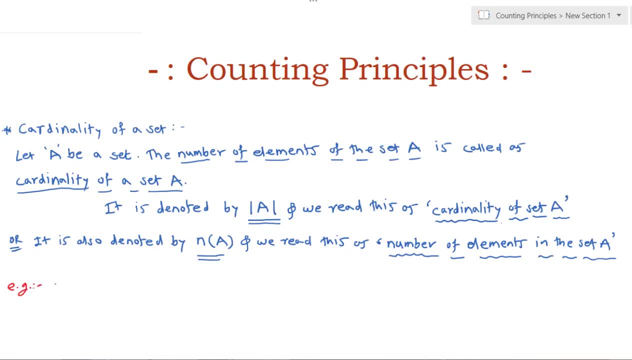 set capital A. Very simple thing. Now I can take some examples. that is, let capital A is equal to A, B, C, D, E, F. Okay, Therefore, cardinality of the set A means two vertical lines and A Cardinality. 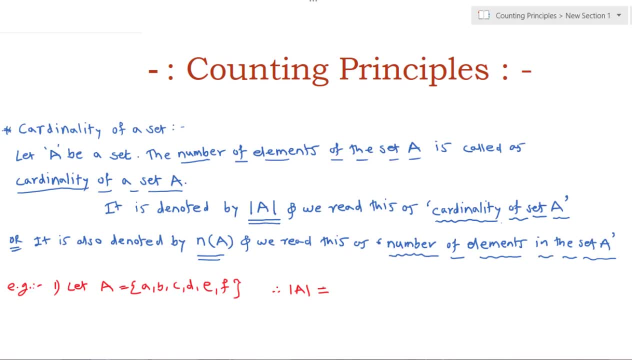 of set A is equal to. what do we have to do? Count the number of elements. Count the number of elements, and the number of elements means the cardinality. How many elements are there? 1,, 2,, 3,, 4,, 5, 6.. Okay, There are 6 elements in the set capital A, Therefore cardinality. 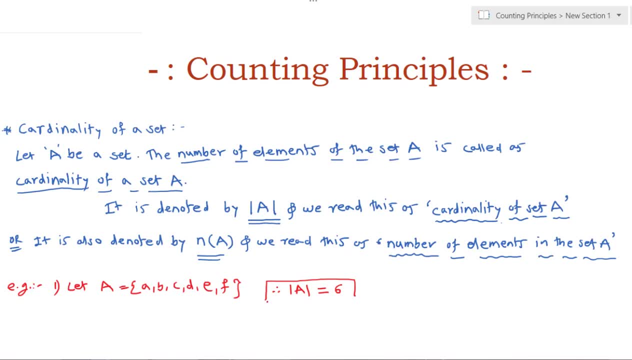 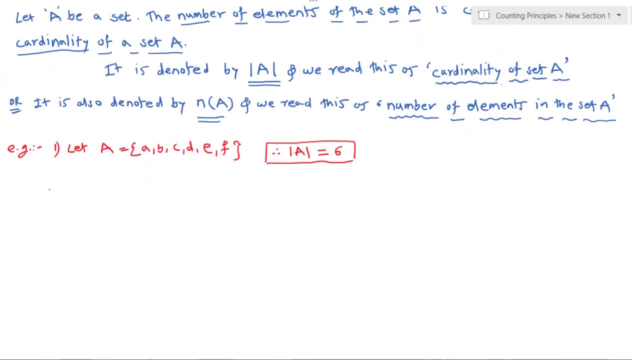 of the set, capital A is equal to 6.. Okay, Very simple thing. Now next one. Let us see another example, Very simple concept. If I consider another example, that is, let capital B is equal to set of all those elements X, such that X belongs to capital N and 2 is less than or equal to. 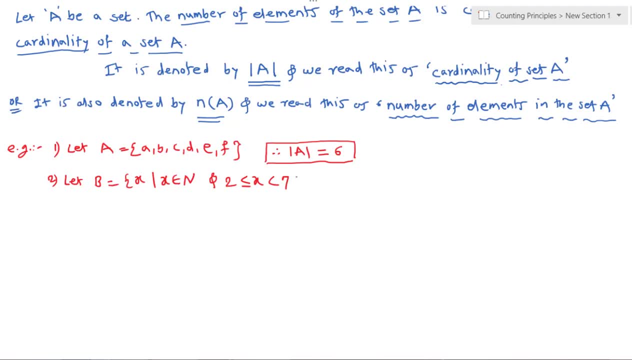 X is strictly less than 7.. Let B is equal to set of all those elements, X, such that X belongs to N and 2 less than or equal to X less than 7.. Okay, Therefore we have to write the cardinality of this set. To write the cardinality first. 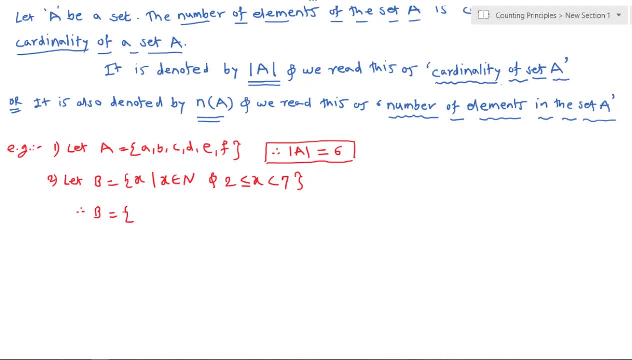 we have to write the elements in the set. Which elements are there? Therefore B is equal to Yes. If we have to put X elements in B, then what is the first condition? X belongs to N. What is N? N is nothing but the set of all natural numbers, Means X is. 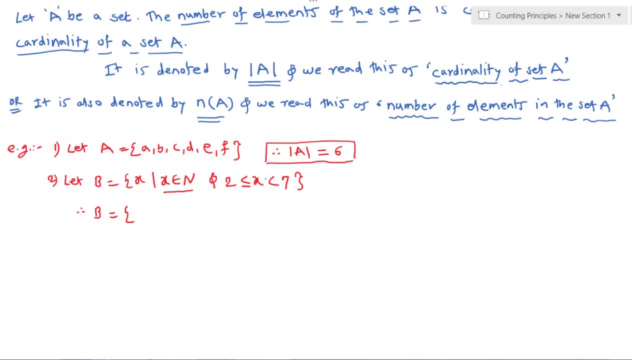 not the only number, It is a natural number. What is X, 2 less than or equal to X less than 7.. Means 2 or 2 is bigger than 7 and 7 is smaller than 7.. Means in B: which elements. 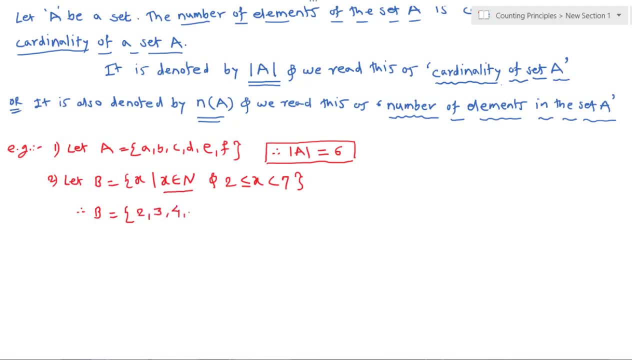 will be given 2 less than or equal to X less than 7.. So B is equal to X less than 7.. And then we have to write it here. So the set of parts are 2 less than or equal. 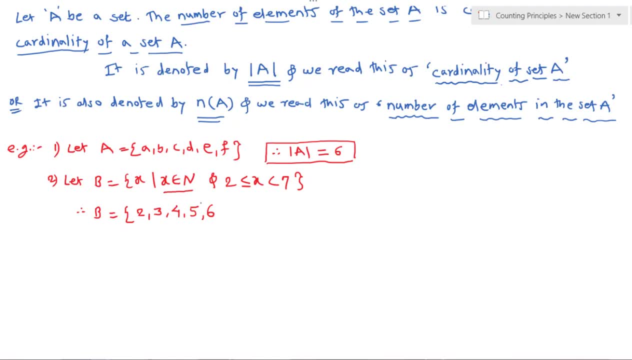 to X less than X less than 7.. What is X less than or equal to X less than 7?? Itarı kalau ki B less than or equal to X less than 7.. That means the number of items in B is less. So if we write it up in B will help in finding this. We have to write this. So X is equal to X, less than or equal to A. B is equal to A, So we have to write it up as a set of. parts. So if I write it up as X less than or equal to A, B is equal to A, B is equal to X less than or equal to B. So X minus 12, a or만 C minus 12, a or a is equal to. 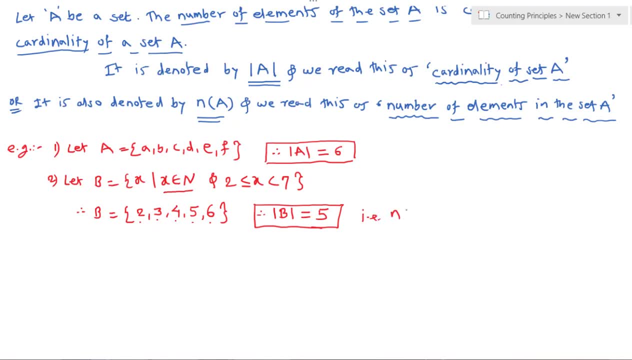 that is n of b means number of elements in the set. capital B is equal to phi yourself. Okay, dhunisa, meaning same as I said, that is the definition of a cardinality of the set. If I consider another example, let c is equal to set of all those element x, such 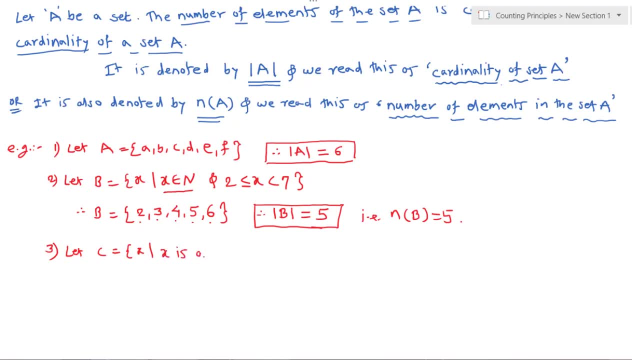 that x is an even number, even number not divisible by 2, not divisible by 2.. Okay, from the high x set we get, c is equal to set of all those element x, such that x is an even number not divisible by 2.. Okay. 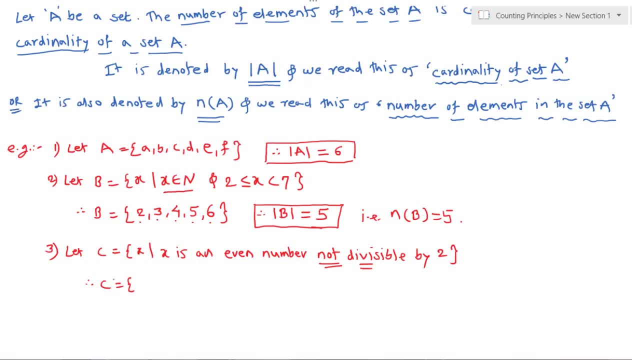 all those elements are. divided means if we want to put all those elements in c, then the condition is: x is an even number. it should be an even number not divisible by 2. How many elements will come? Which element will come? Yes, even one element will not. 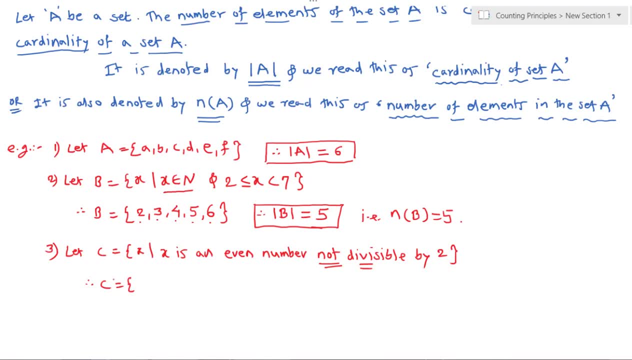 come in this because we know that every even number must be divisible by 2, every even number should have two parts. even number which does not have two parts should not exist in the existence means even one element will not come in c. that is, c is equal to empty. 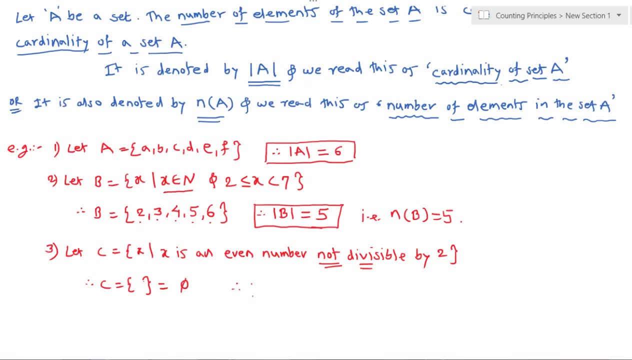 set of cells, phi of cells. Okay, therefore, cardinality of c is equal to number of elements in the set capital c. c is not even one element means, of course, cardinality of c is equal to zero cell. getting this: 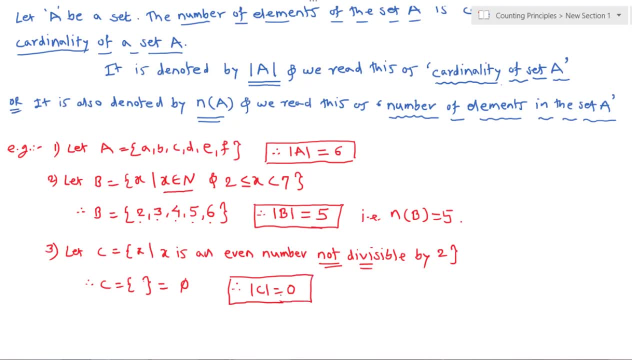 Okay, very simple thing: cardinality of c is equal to zero cell. cardinality of c is equal to phi, not zero cell. that is the simple concept of cardinality of the set. Okay, now, next one. we have to see some principle, that is, counting principles, counting principles. 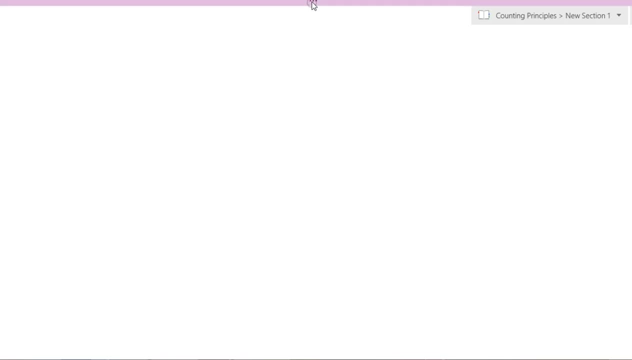 okay, Let us see some principle, out of which let us see the first principle: Counting 실천 princiプль, counting principles, counting principle of 1, that is ein edition principle. edition principle. Okay, very simple thing. New book of principles. let capital A and 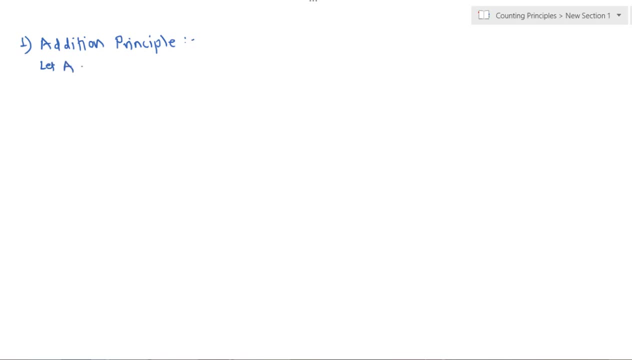 capital B be count countante principaleszuf, mirroring principle, countante principal capital A and capital B, B, B, E, any two disjoint sets, any two disjoint sets. then we have then addition. principle states that then we have cardinality, of A union with B. 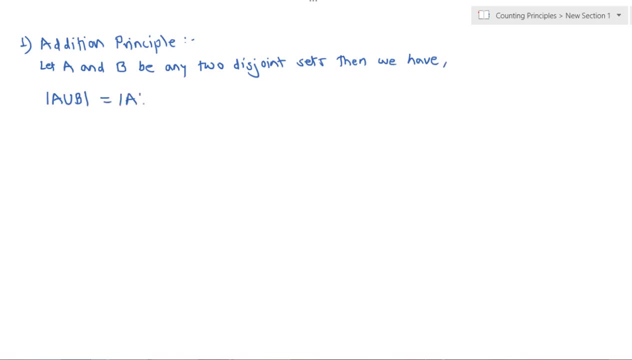 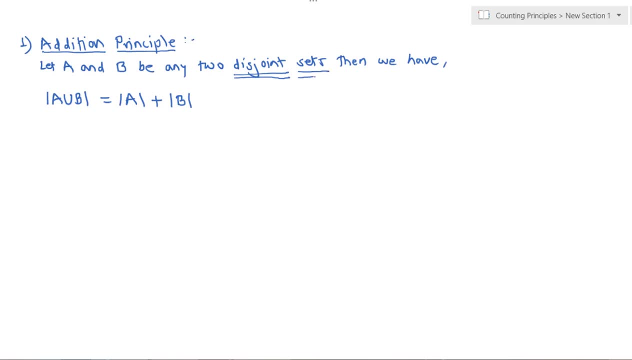 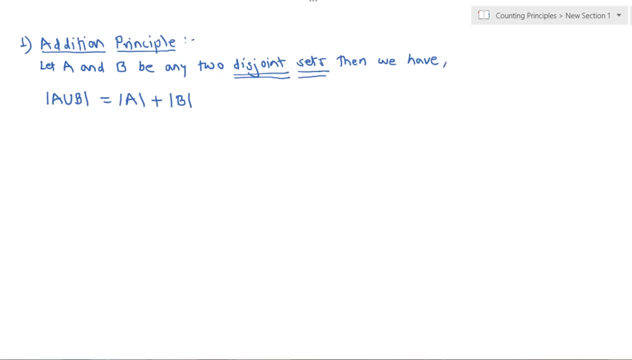 two disjoint sets. then we have: cardinality of a union b is equal to cardinality of a plus cardinality of b, sl. okay, when you set a and b quantity, don't say it is still the cardinality of a union b is the card i choose. ali, the principle might not last the kai. 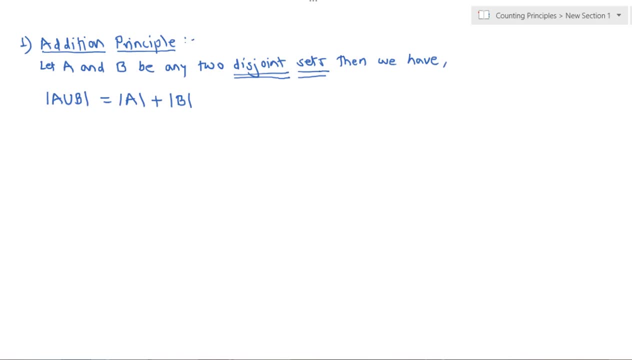 have to do, set a set b from a union b, which set have to do, and set a union b after taking out a union b. in that set, number of elements have to be counted. number of elements mean the cardinality of that set. ha, what is the advantage? what is the number of elements in? 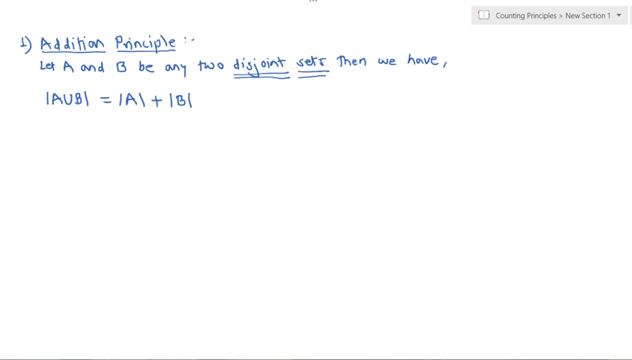 b and how many in a. you might know the number of elements in b. you might know it definitely without finding the elements in the set a, union b, we can starts the cell and warm up will be played a common word in the set b because if we have one number of elements we can say a and b have a different finesis. 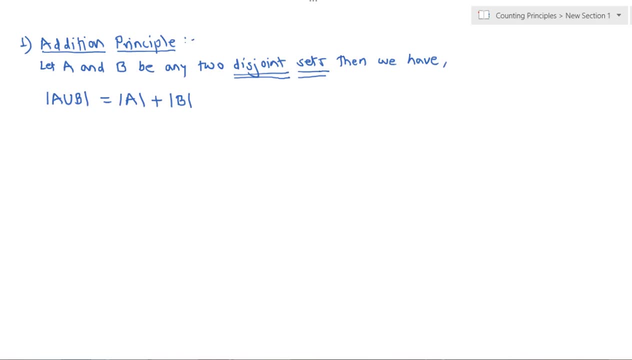 can find the cardinality of the set A union B. getting this okay: A union B, your set elements, elements, cardinality. that is the advantage of this particular addition principle. okay, very simple thing. let us see another principle, principle number 2, that is a multiplication. 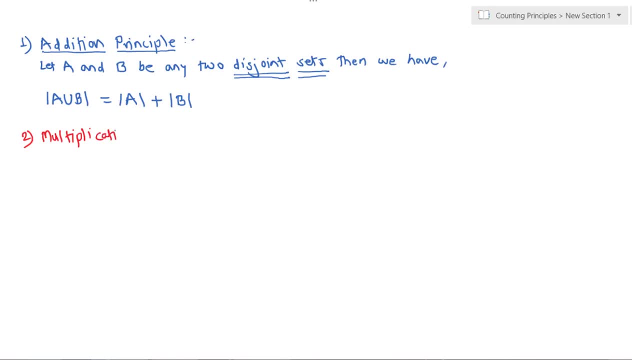 multiplication, multiplication principle. multiplication principle- okay, what is that? very simple thing. let capital A and capital B. let capital A and capital B, B, B, E, any two, any two finite sets, any two sets. then then we have then multiplication principle. 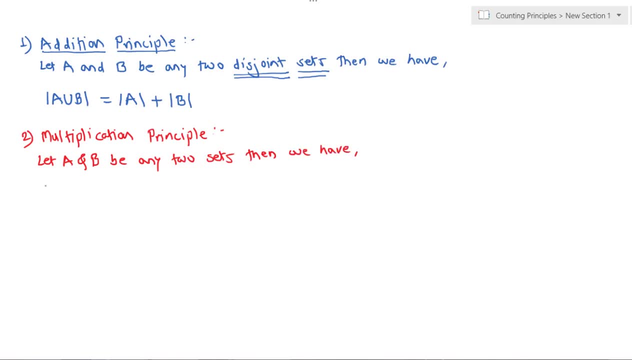 principle states that then we have comma. next line: cardinality of A cross B. cardinality of A cross B is equal to cardinality of A into cardinality of B. okay, simple concept, simple principle, multiplication principle: let A and B be any two sets, finite, infinite. 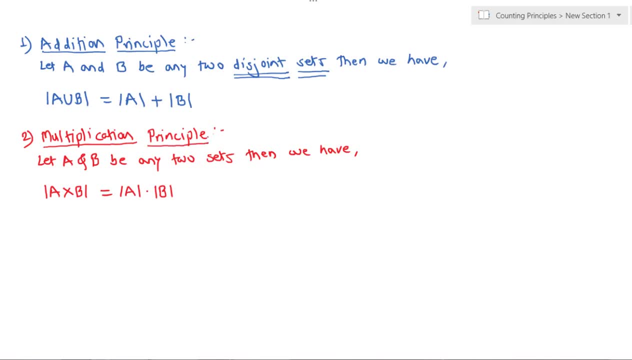 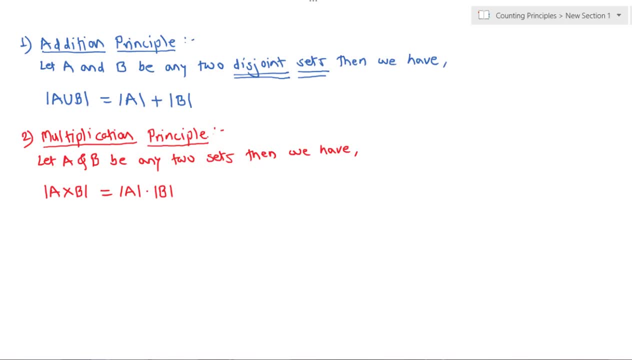 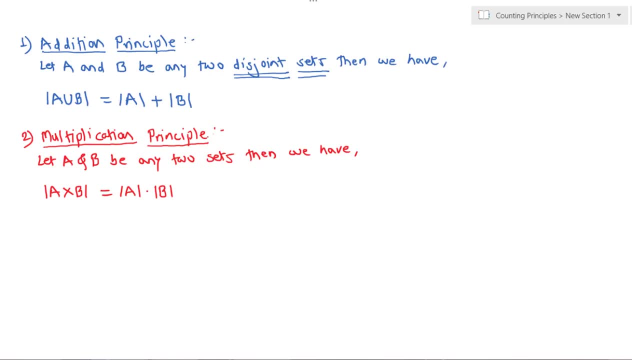 The computation product of A with B. how many elements are there? 5 into 3 is equal to 15 elements are there. That is the simple multiplication principle. Getting this Okay, Very simple thing. Now we have to see third principle. 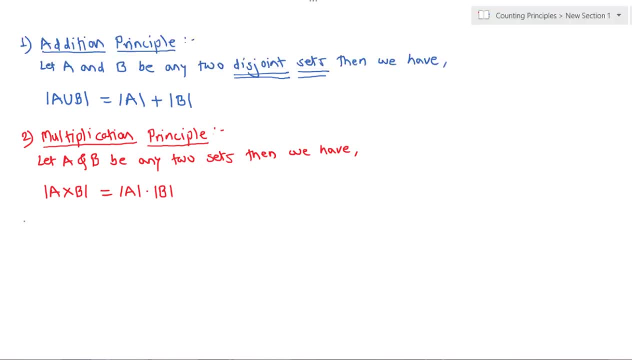 We can also prove all the principles, But only the principles need to be known. Okay, Third principle: Now let capital A and capital B be any two sets, Be any two sets. Then we have cardinality of A minus B. 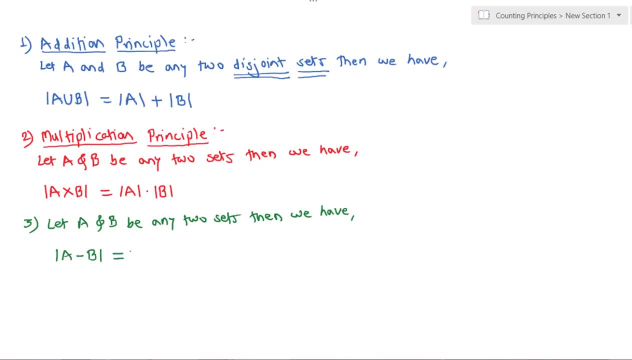 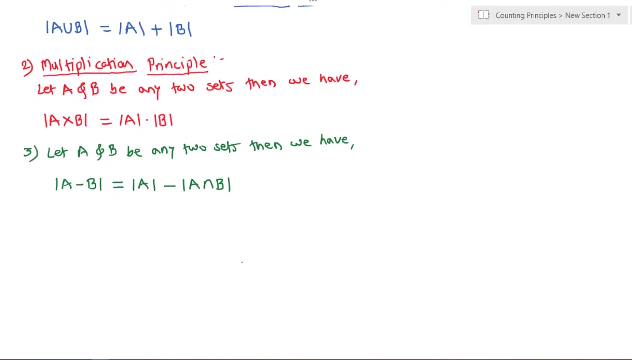 Cardinality of A minus B is equal to cardinality of A minus cardinality of A intersection with B. Okay, So that is the simple multiplication principle. Okay, Simple concept: A and B are any two sets. Then we have: cardinality of A minus B is equal to cardinality of A minus cardinality of A intersection with B. 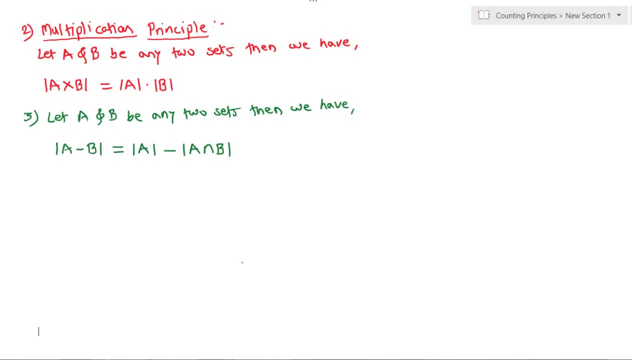 Getting this Now: A minus B. What does it mean? These are the set: A is set, B is set. A minus B has only set. A intersection: B has only set. It means in the set theory all the operations are there. 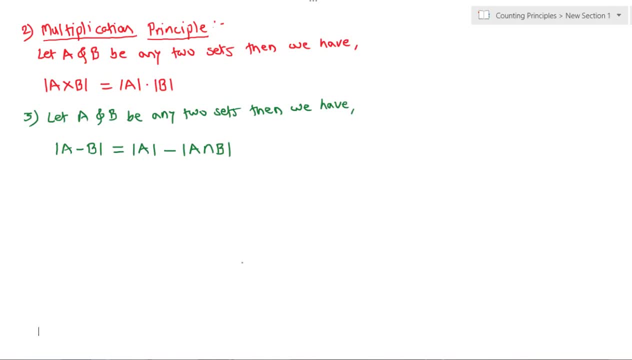 And the operations of the set theory that you know very well. Okay, These are basic concepts. Cardinality of A minus B is equal to cardinality of A. Cardinality of A minus B is equal to cardinality of A intersection with B. 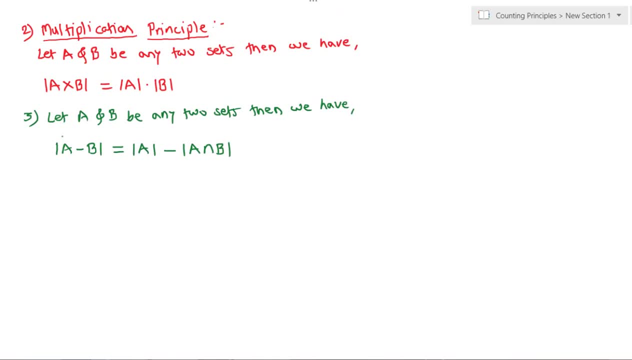 Okay. So what is A minus B? Set of all those elements which belongs to A but does not belongs to B. Okay, That you know very well. A intersection B is set of all elements which belongs to both A and B. Okay, 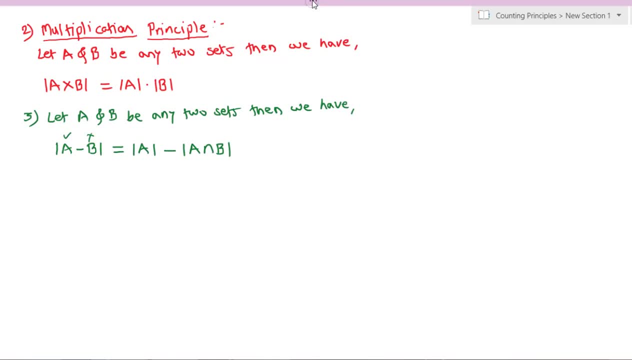 That is the principle: Cardinality of A minus B is equal to cardinality of A minus cardinality of A intersection with B. Okay, Let us move towards the next one, Fourth principle, Which is again very important principle. Name of that principle is a principle of: 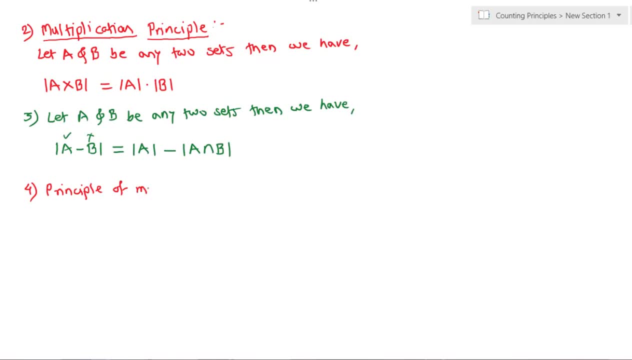 Principle of mutual inclusion: exclusion. Mutual inclusion- dash comma slash. exclusion for two sets: Okay, For two sets. For two sets Okay. Don't say it is a principle of mutual inclusion exclusion. Very simple thing, Atisha. so far I have a statement book. 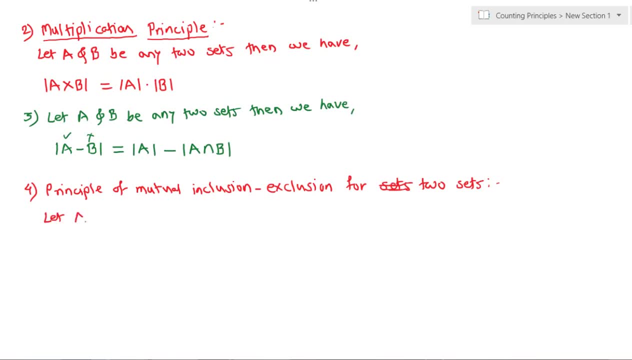 Okay, Let capital A and capital B, B, B, E, any two sets Then Then Then we have What then? The principle of mutual inclusion- exclusion for two sets- states that asamalata is all. Okay. Then we have very simple thing. 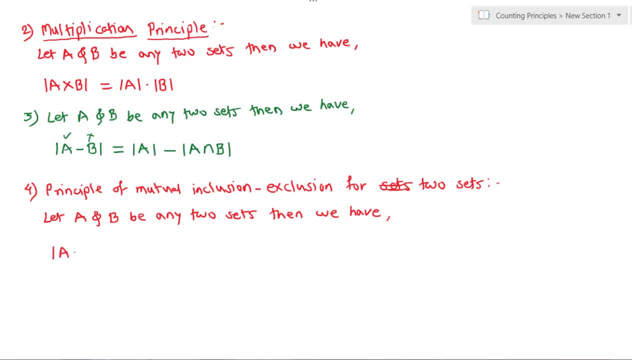 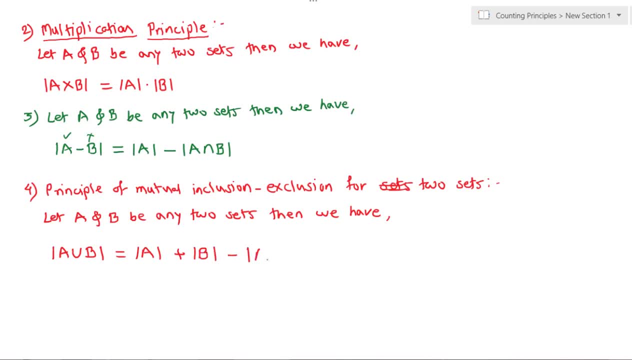 So, let us see, So, let us see, So, let us see, minus cardinality of A intersection with the B. Simple thing: cardinality of A union B is equal to cardinality of A plus cardinality of B, minus cardinality of A intersection B. 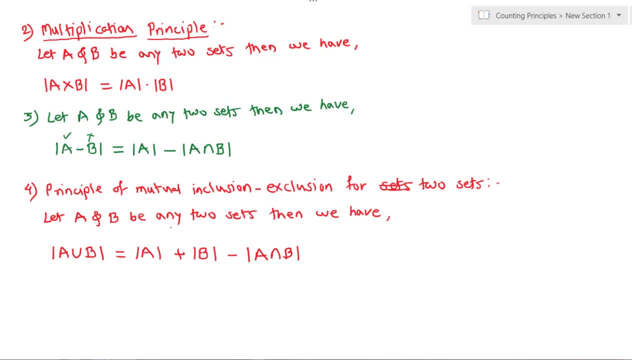 Kaya statement de puna ekta bhogiya. let capital A and capital B be any two sets, Konte hi don sets aahit. Then the principle of mutual inclusion- exclusion for two sets- states that cardinality of A union with B is equal to cardinality of A plus cardinality of B minus. 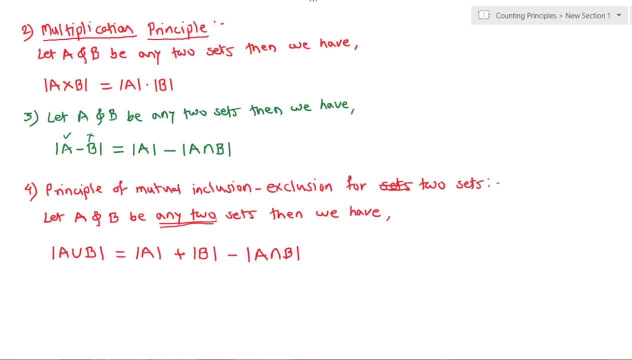 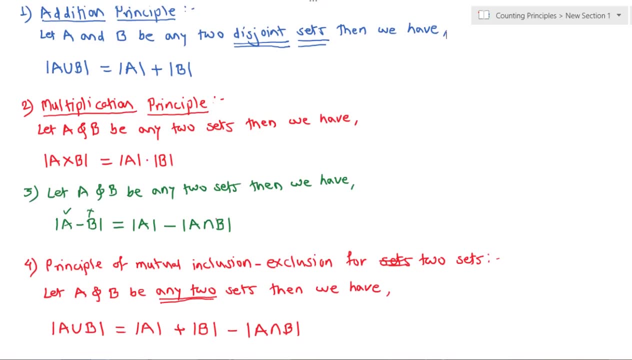 cardinality of A intersection with the B. Now, if we notice our principle number 1, that is the principle addition, principle, Addition principle, ma de sudha LHS. kaya bhagavar LHS. is the A union B. Similarly, principle of mutual inclusion: exclusion- ma de sudha LHS. 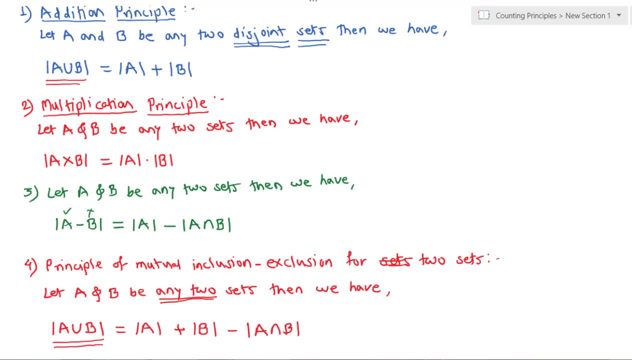 kaya hai A union B, hai Tika of A- union B. In addition, principle: there is LHS Carnality of A plus Carnality of B and principle of mutual inclusion: exclusion for two sets: there is LHS Carnality of A plus Carnality of B minus Carnality of A. intersection with: 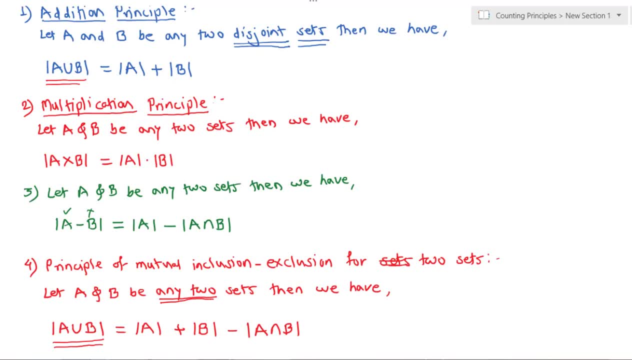 B. Both have same LHS, but LHS is distinct When to use addition principle and when to use principle of mutual inclusion- exclusion For that let us see the conditions. Addition principle we can use only when the two sets are disjoint sets. 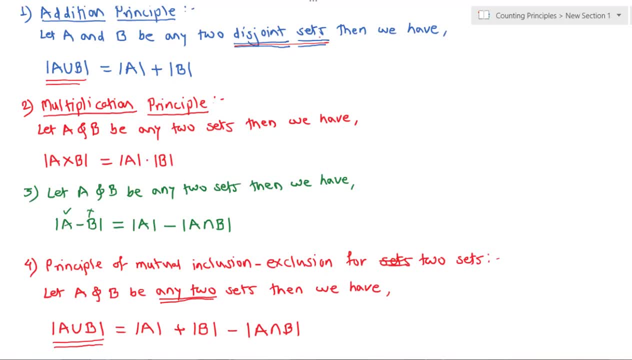 Also, if there are two sets are disjoint sets, then A and B may not be common. Then addition principle is used In principle of mutual inclusion, exclusion. any two sets- A and B means may be disjoint, may be not. Any two sets may not be common. 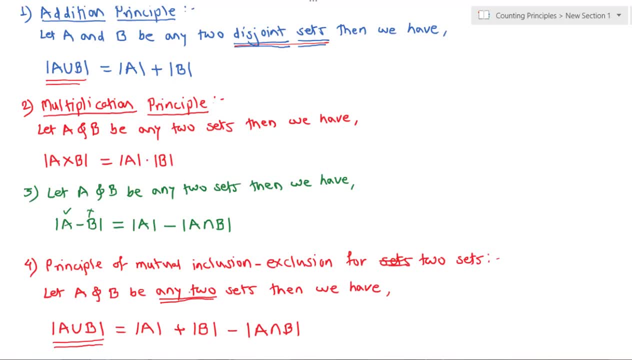 wellness. means principle of mutual inclusion, exclusion that is, which can be applicable anywhere but the addition principle is a particular principle which can be applicable only when the given two sets are disjoint sets. means principle of mutual inclusion exclusion is a general case, while the addition principle is a particular case of. 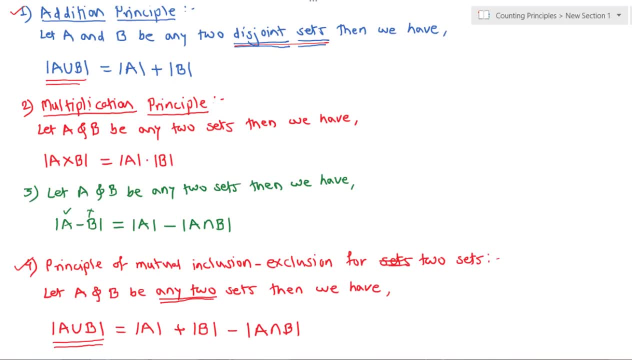 principle of mutual inclusion, exclusion for two sets. giving this, then, what is disjoint sets? here and there, disjoint sets means what A intersection B is equal to 5, then what about its cardinality? therefore, cardinality of A intersection B is equal to 0. 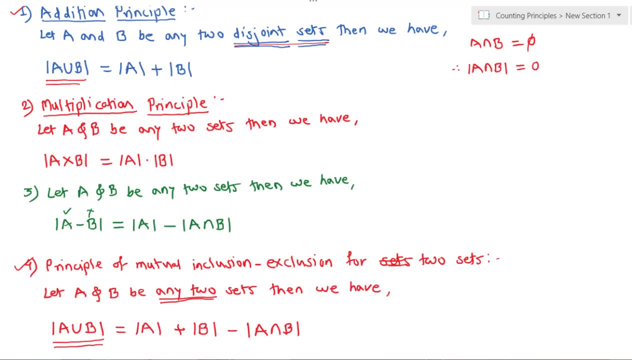 means A and B are disjoint sets. then A intersection B cardinality is 0 and then ether principle of mutual inclusion, exclusion means A intersection B cardinality is equal to 0. then cardinality of A union B is equal to cardinality of A plus cardinality of B minus 0. 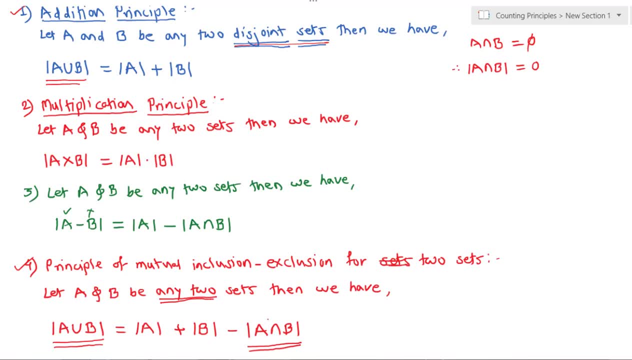 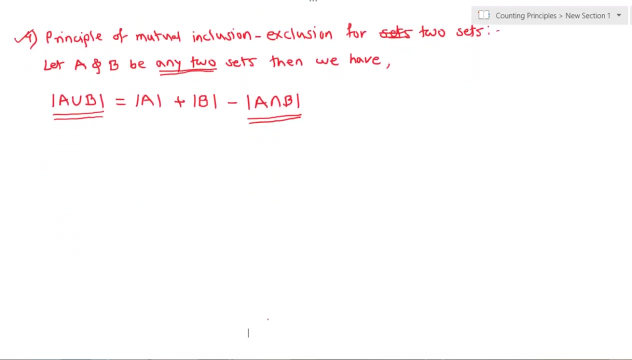 means we get addition principle. getting this means principle of mutual inclusion, exclusion for two sets. these are the general principle, and to that general principle we have put condition. what condition to put? A and B are disjoint sets. these are the condition we have put. then what will we get? 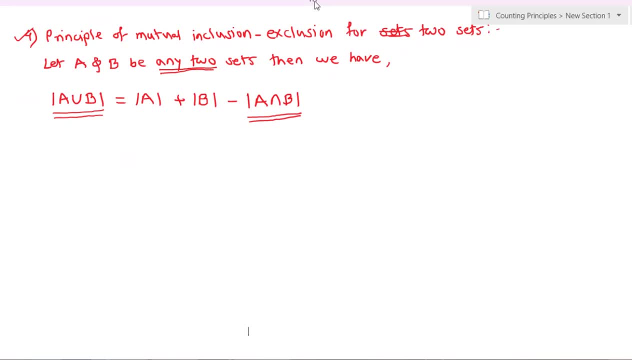 yes, addition principle- we are getting. this means addition principle is a particular case of a principle of mutual inclusion exclusion for two sets. number 5 possible principle, last principle, that is, a principle of mutual inclusion exclusion. mutual inclusion, dash exclusion. dash exclusion for three sets, for three sets a top and don't set sati. principle of mutual inclusion exclusion. 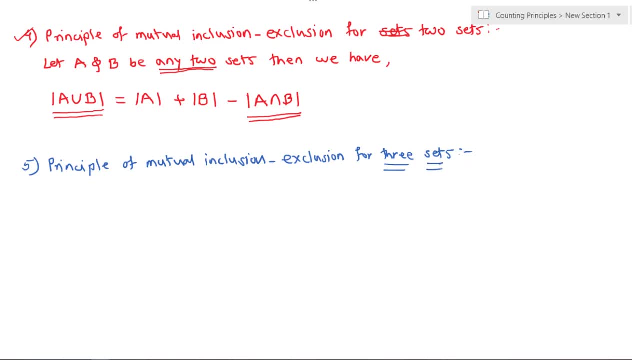 Kyber, Hitler, other, that's the extension for three sets: kill alive. okay, Kyra, gap, don't set sati the site, the sustain. set sati. let capital a, capital B and capital C be any three sets, any three sets then. then principle of mutual inclusion: exclusion for the three sets states. 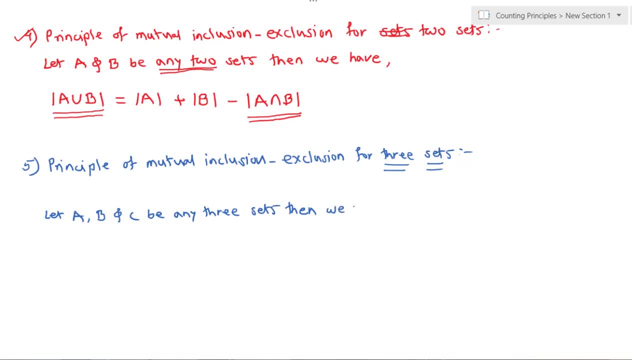 that, as a man later, is a little. what then we have? then we have I principle everywhere, very simple thing: cardinality of a union with the B, union with the C, is equal to very simple statement: cardinality of a plus cardinality of B plus cardinality of C. 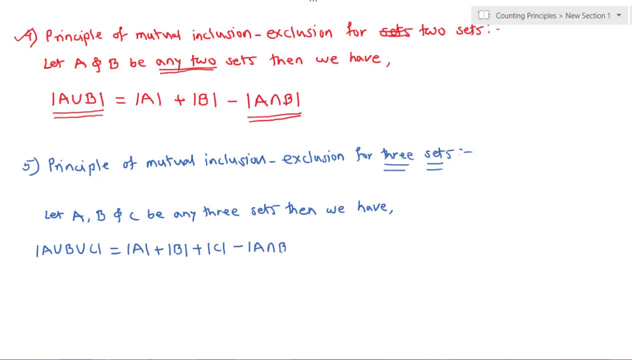 minus cardinality of a intersection with the B, minus cardinality of B intersection with the C, minus cardinality of a intersection with the C, plus cardinality of a intersection with the b intersection with the c. okay, very simple thing. this is the principle of mutual inclusion. exclusion for three states. 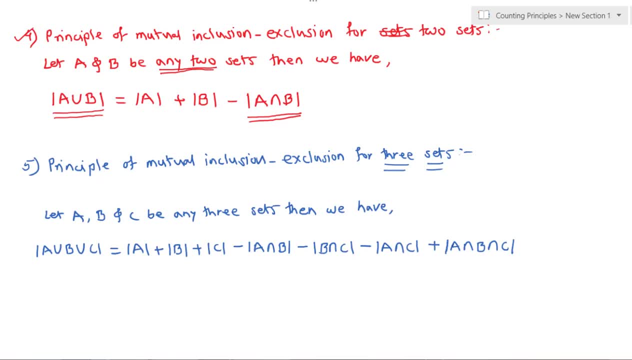 how to remember this principle. karnality of a union b union c is equal to karnality of a plus karnality of b plus karnality of c. okay, that is very simple. put it: minus, minus karnality of a intersection with the b. 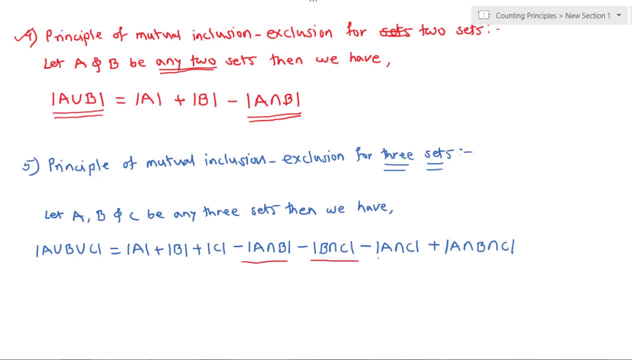 minus karnality of b- intersection c. minus karnality of a intersection with the c. okay, cyclic bhaja a, b and c: okay. minus karnality of a- intersection b. minus karnality of b- intersection c. minus karnality of b- intersection c. 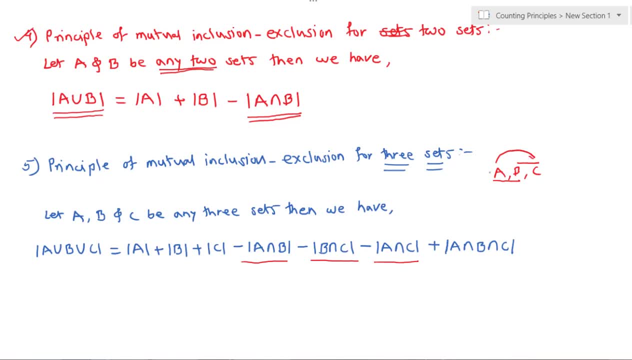 minus karnality of b intersection c, of a intersection with the same- and your pilot is not okay- a, b, b, c, c, a, c, a, mana, q, y, a, c, mana, current intersection c and c intersection a same as i, that you know very well- minus continuity of a intersection c and plus tighanchi intersection, waza kava. that is a plus, sorry. 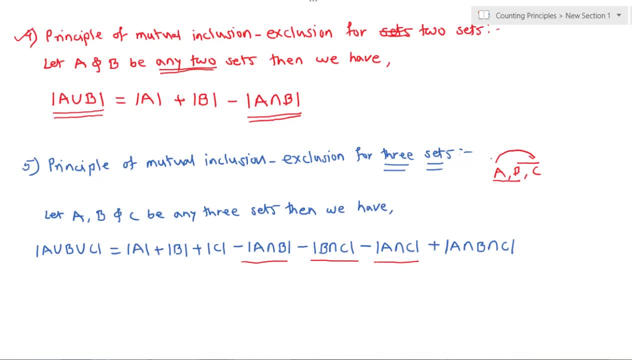 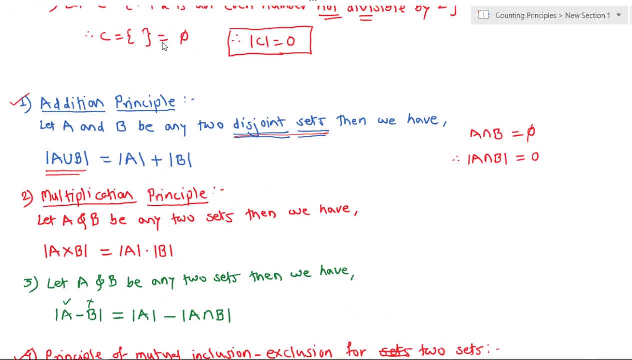 plus kava, plus continuity of a, intersection with the b, intersection with the c, getting this: this is nothing but the principle of mutual inclusion: exclusion for three sets. okay, okay. this is nothing but the principle of mutual inclusion: exclusion for three sets. okay, okay, okay. So we can see the same thing in number of elements. 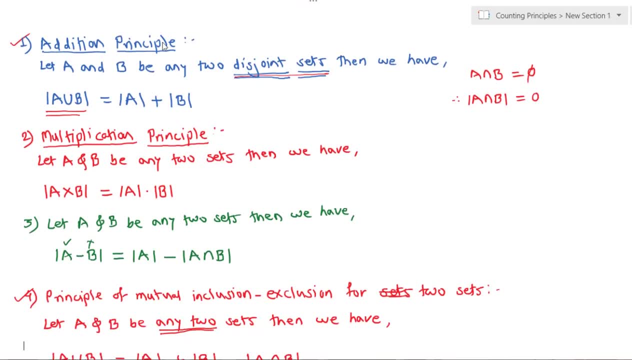 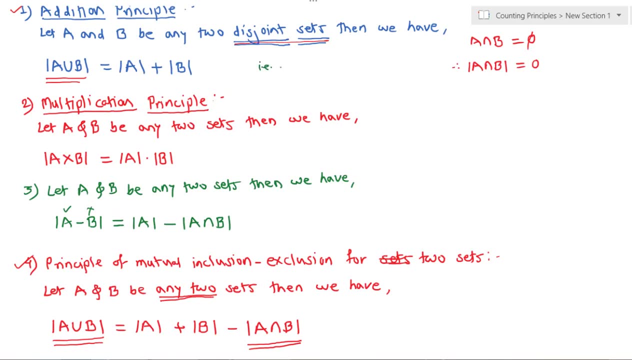 As we discussed earlier, Carnality of A union B equal to Carnality of A plus Carnality of B. This is our addition principle. What is the addition principle N of A union B means number of elements in the set. A union B is equal to. 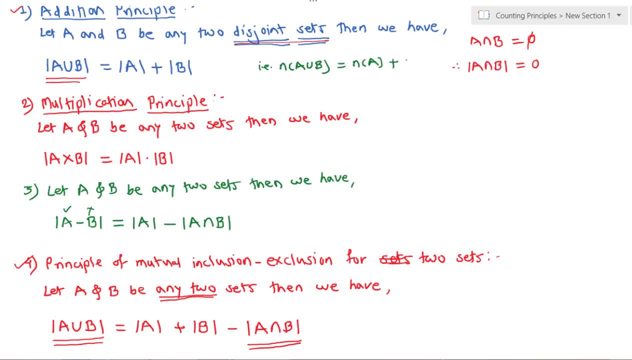 N of A, that is number of elements in the set capital. A plus N of B, that is number of elements in the set capital BSL. Probability in this chapter in statistics paper. probability in this chapter in complete statistics paper. symbol N of set is like this: 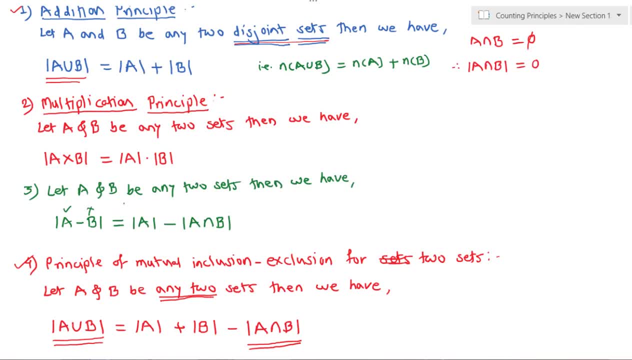 So you need to know this symbol also. Similarly, multiplication principle. what is it? Yes, carnality of A cross B is equal to carnality of A into carnality of B Means number of elements in the set A cross B. 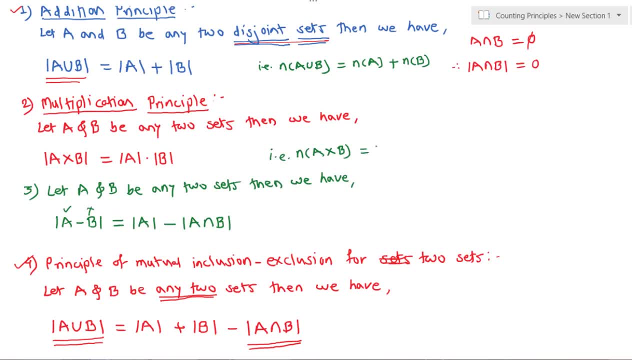 that is N of A. cross B is equal to N of A into dot. N of B. Dot means our name is a product. N of A into N of B. That is number of elements in the set capital A into number of elements in the set capital BSL. 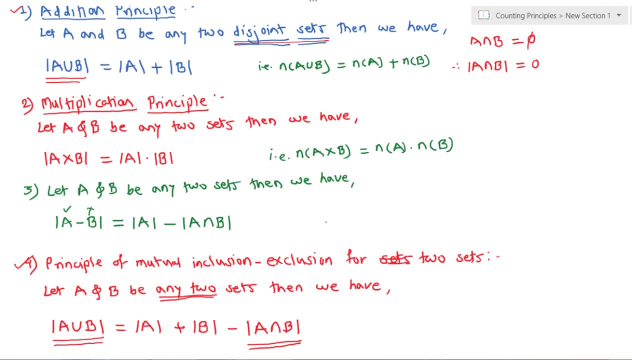 Similarly, this principle- what will be Carnality of A minus B- is equal to carnality of A minus carnality of A intersection B, Means number of elements in the set A minus B is equal to number of elements in the set capital A cross B. 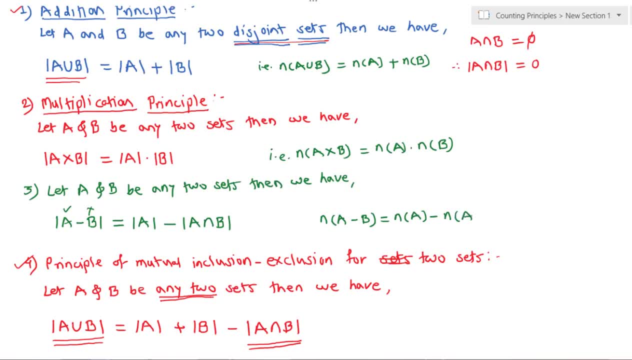 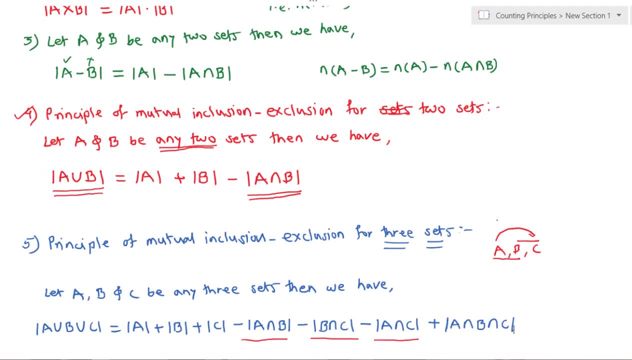 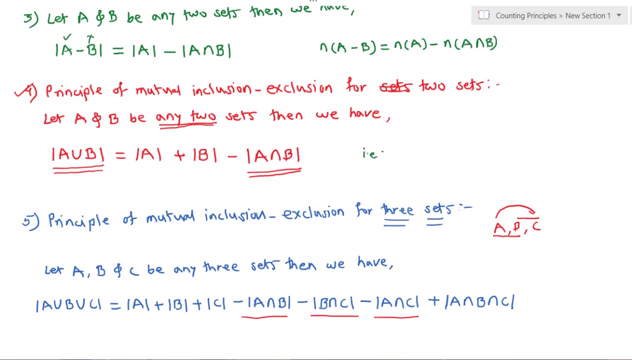 Capital A minus number of elements in the set A intersection with BSL. Simple thing. Similarly we can see principle of mutual inclusion, exclusion for two sets in another. symbols. that is: yes, number of elements in the set A union with B is equal to number of elements in the set capital A. 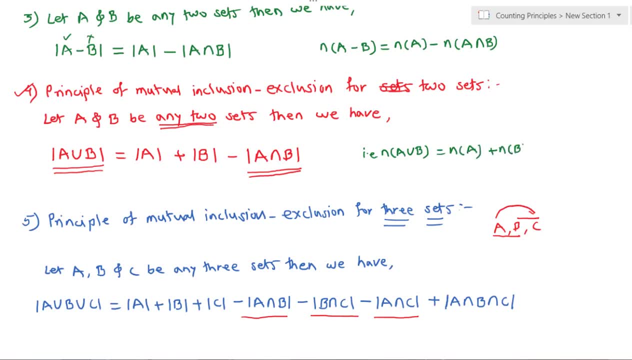 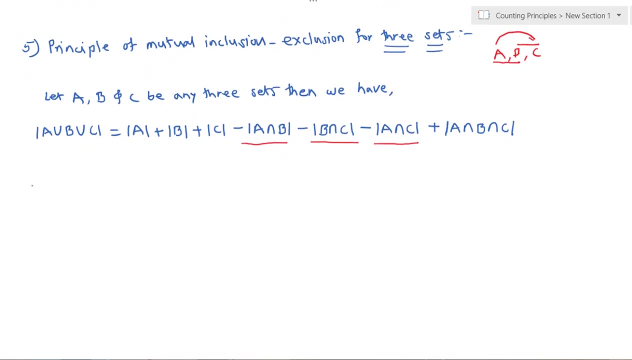 plus number of elements in the set capital B, minus number of elements in the set capital B. Yes, similarly, principle of mutual inclusion: exclusion for three sets. What is that? N of A union with B union C is equal to N of A number of elements in the set capital A. 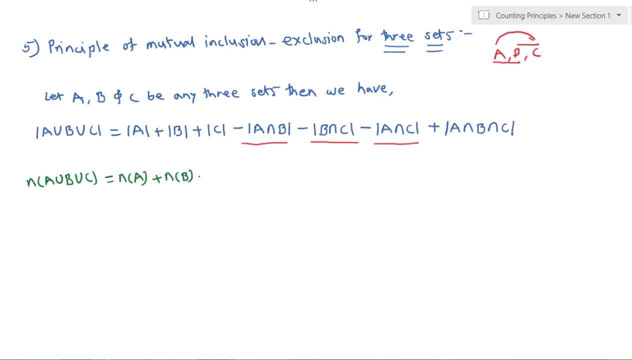 plus number of elements in the set capital B plus number of elements in the set capital B plus number of elements in the set capital B. number of elements in the set capital C minus number of elements in the set A intersection with B minus number of elements in the set B intersection with C minus number of elements.